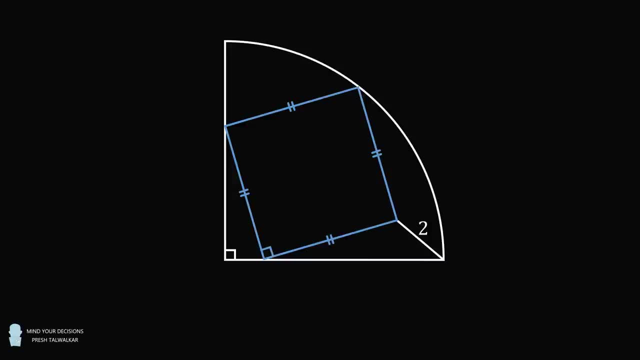 the quarter circle is equal to two. From an adjacent quarter on the radius, the horizontal length to the corner of the quarter circle has a length that's equal to five. The question is: what is the side length of the square equal to? This was posted on Reddit Ask Math with the title: 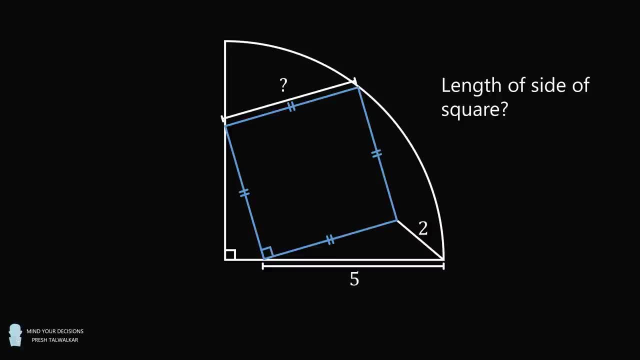 that this problem stumped the entire math department. Now, in order to solve this, you are allowed to give an approximate value to three decimal places. You can use a symbolic or numerical solver. The problem was created by at Dare2Solve on Instagram and Twitter, and I thank Forteleza and Wally for the suggestion. 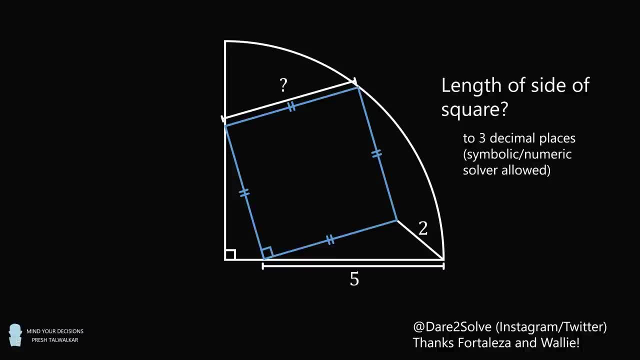 Pause the video if you'd like to give this problem a try And, when you're ready, keep watching to learn how to solve this problem. To solve this problem, we will construct some triangles. Drop a perpendicular right here and say: this side length is equal to b. Then let the other 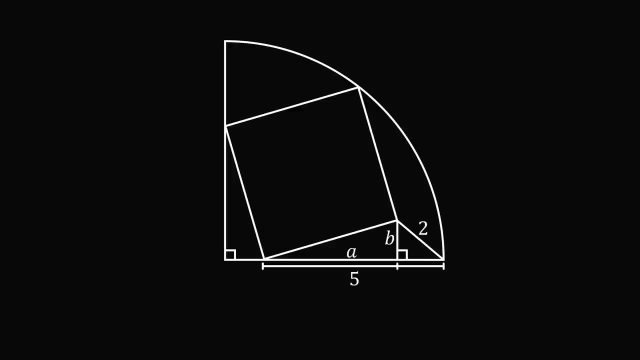 leg of this right triangle be equal to a. So then this length of five will be equal to a and five minus a. This right triangle with legs of a and b is exactly congruent to the right triangle that's on the center of this quarter circle. So this right triangle will have legs of b and a. Now 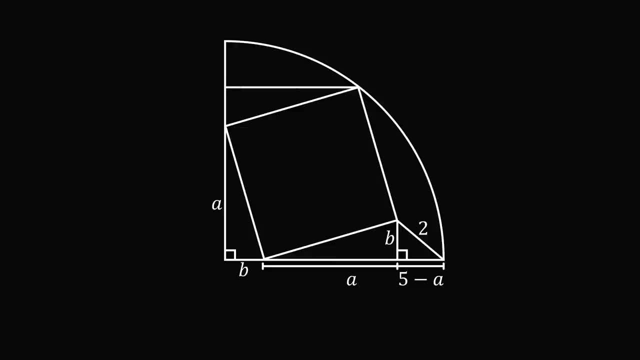 we'll construct another congruent right triangle by dropping a perpendicular from the corner of the square right here. So this right triangle will have side lengths that's equal to b and a. Construct this radius of the quarter circle. Now, the radius of the quarter circle will be: 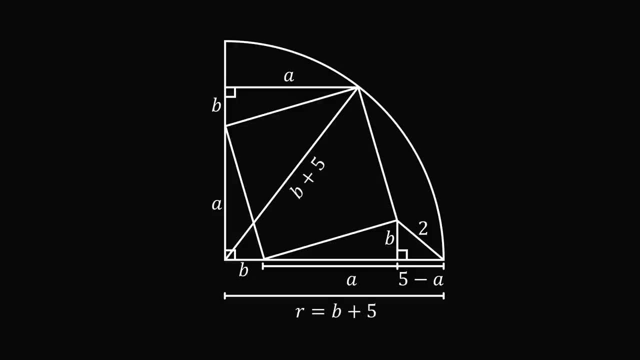 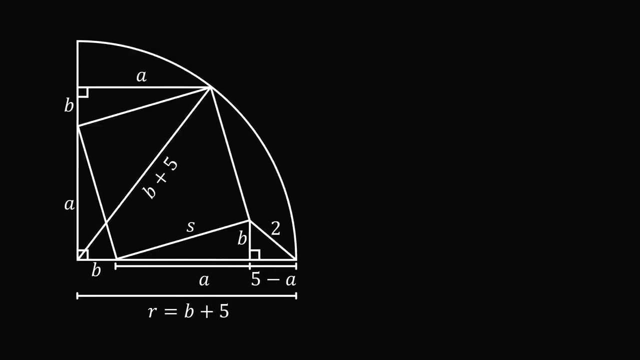 equal to b plus five. So this length will be equal to b plus five. So now we're pretty much ready to solve the problem. Let the side length of the square be equal to s. Now in this right triangle we have a plus b. the quantity squared plus a squared is equal to the square of b plus 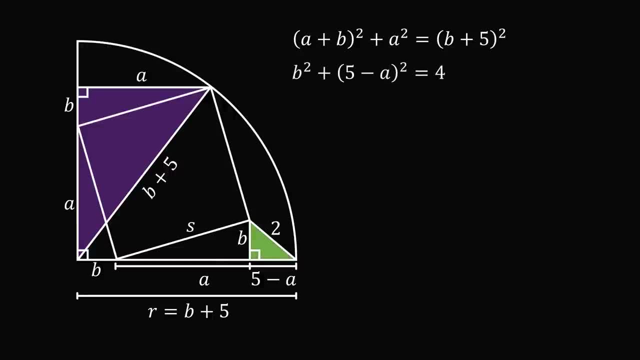 five. In this right triangle here we have b squared plus, the square of five minus a is equal to two squared, which is equal to four. So in this right triangle here we have a squared plus b squared is equal to s squared. Now you could work through these equations. You'll end up with a quartic equation in a.